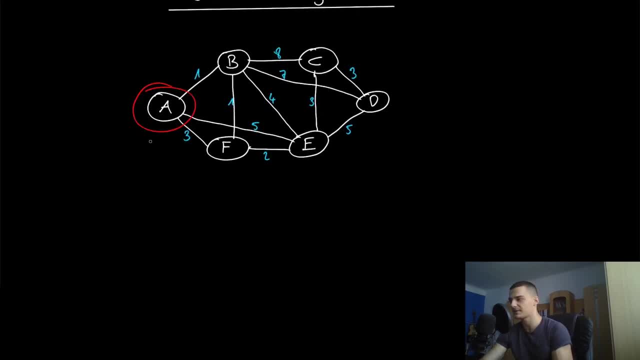 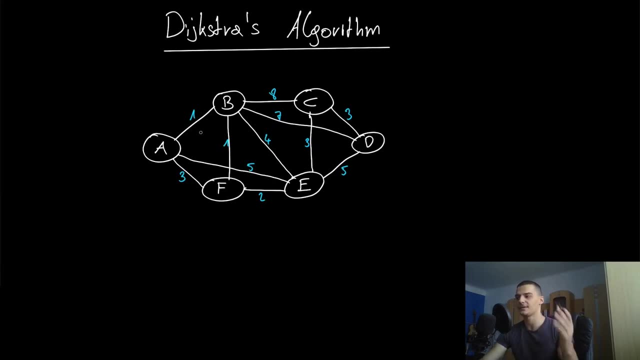 A to any other node. This is what a Dijkstra's algorithm does. We pick a starting node- in this case A, and applying the Dijkstra's algorithm, what we get is the shortest path from A to any other node. We don't have to select a specific target node, it just gives us all the 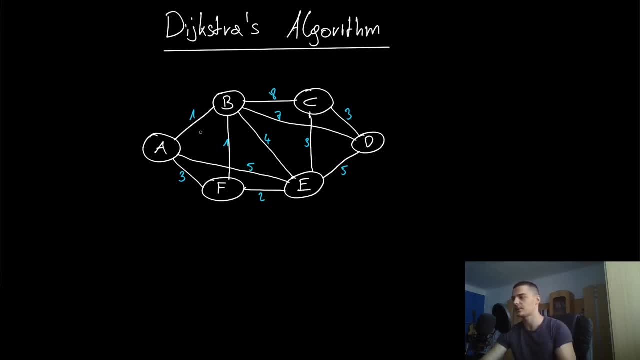 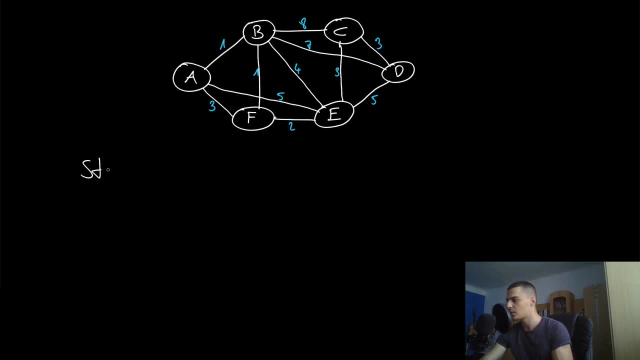 shortest paths from A to B, from A to C, A to D and so on. And what we need to do in order to apply the Dijkstra's algorithm is we need to set up a table here with one column, which is called step. 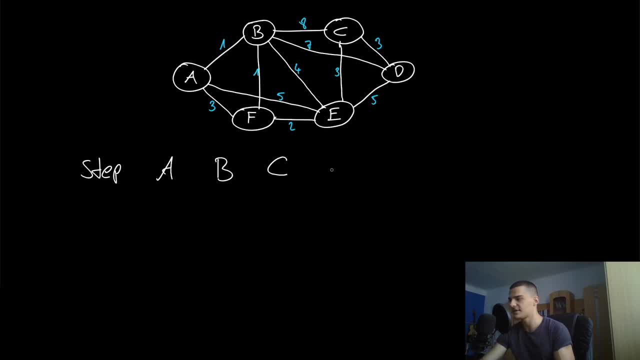 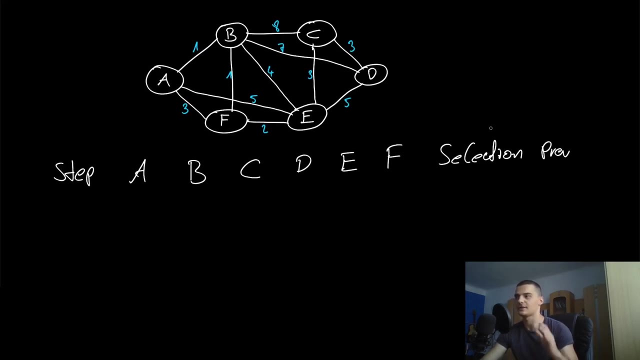 then a column for A, for B, for C, for D, for E, for F, and then two more columns. One is the selection and one is the previous node. Now, the Dijkstra's algorithm is not complex at all. It's a very 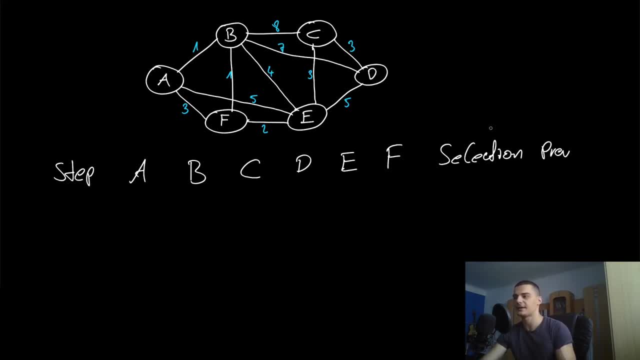 simple, very intuitive algorithm. It's easy to understand. We just need to fill out this table here in a very simple manner. So we choose a starting point, in this case A, and what we'd write down is, with one step, how much. 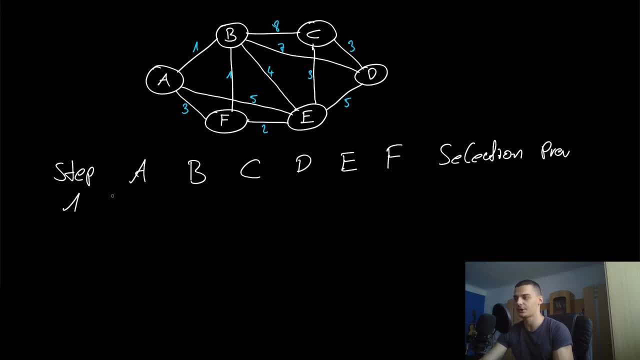 distance is there from A to the other nodes. Now we can ignore this column here, because A to A is zero or nothing. actually We cannot say zero, because otherwise we would have to select it. Or we could say, with zero steps it's zero, so select it, and so on. But essentially what we do is we write down the 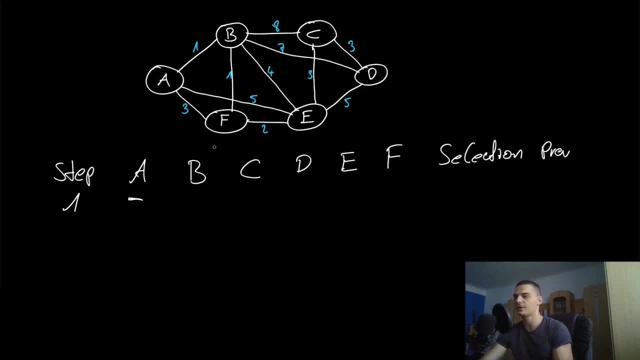 cost of going from A to all the other nodes using one step. One step meaning that we can use one edge. So in this case, from A to B it's one, from A to C it's infinite. because I cannot. I don't have a direct connection between A and C, but I only have one step, so I cannot go. 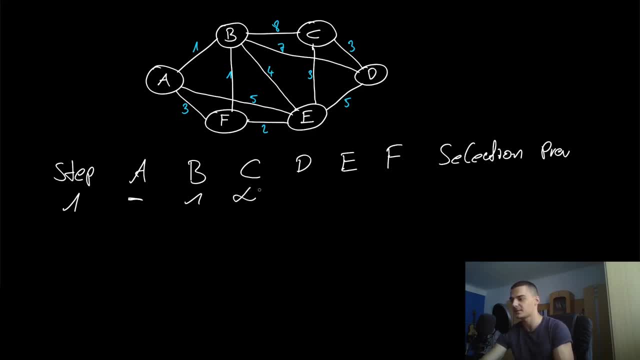 A, B, C. I have to go directly there and this is not possible. so we're going to say infinite: From A to D, it's the same thing, and from A to E I have a cost of five, and from A to F I have a cost of three. Now, the simple thing here that we need to do in the 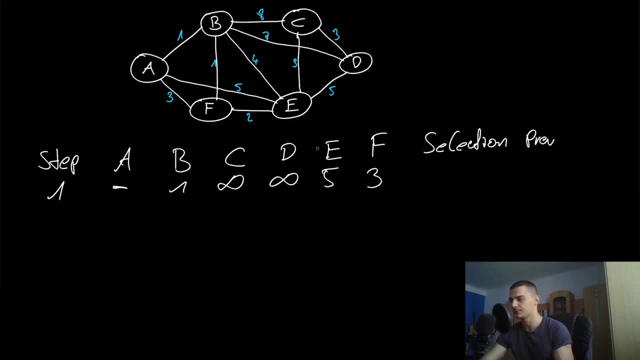 Dijkstra's algorithm is we just select the smallest value. Very trivial: the smallest value that we have here is one, It's the connection from a to b. And then what we do is we just say: okay, we select b and we write down. 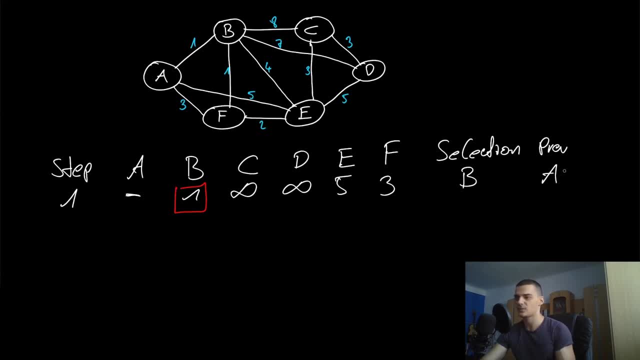 where we got from, where we got to B. So in this case, A was the previous node, so we got from A to B, and this is the selection. Now the next step is looking at two-steps. So now we're looking at how. 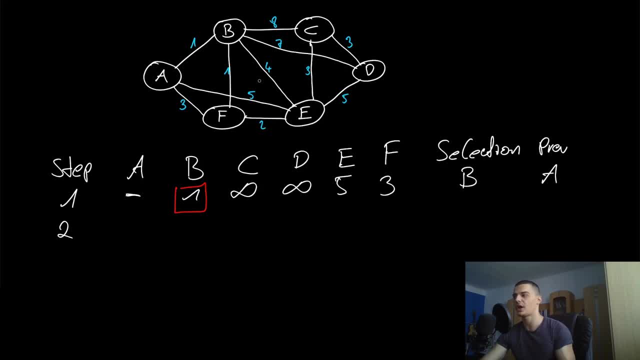 much does it cost to get to a certain node using two-steps- And we're not looking at all the two-steps possible- going to see or to check what is the cost from a to e and then to d, or from a to e and then to c? 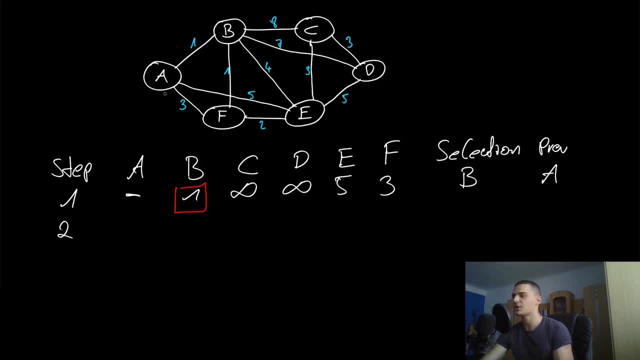 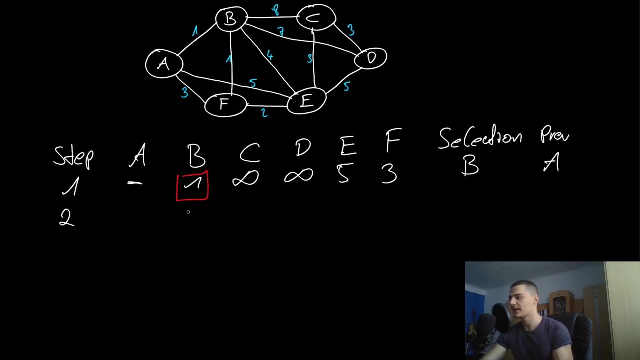 or from a to f and then to b, and so on. we're just going to look one more step from the note that we selected. so we selected b, and now the only thing that we need to do is: what can i reach using one more step from b? and then, of course, we need to add the cost here, so in this case, we could go ahead. 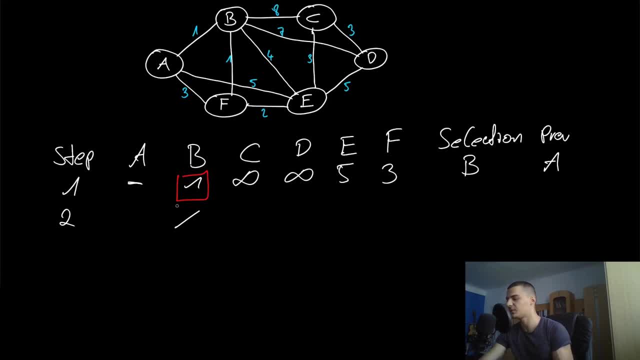 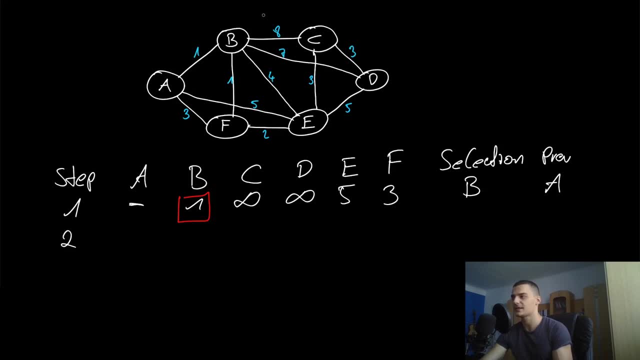 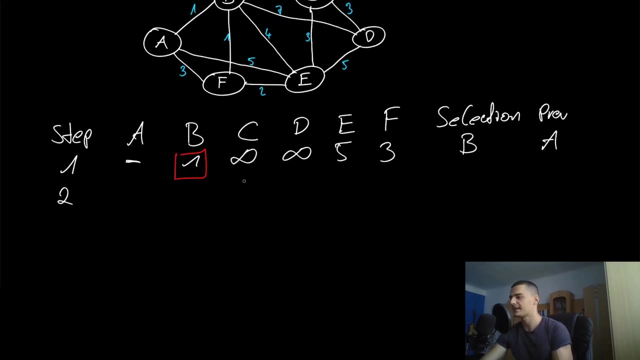 b is now that we don't care about b and we don't care about a. we ignore these two, um, and we now ask: okay, how much does it? uh, how much does it cost to go from b to c? it costs eight. so going from a to c costs one plus eight when we go through b. so we write down: uh, nine, so it's one plus eight. 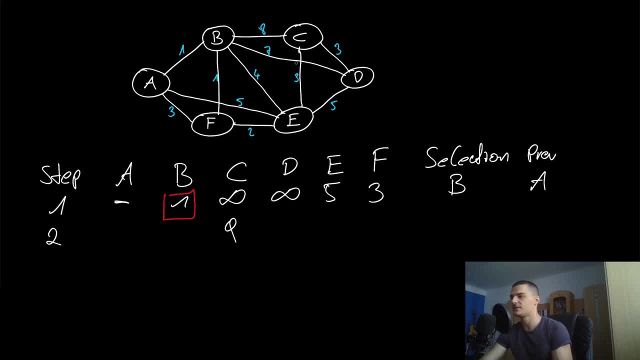 it's nine. um. and then the next thing is going from a to d. going from a to d is one plus seven, so we have a cost of eight. now, going from a to e is the same with one step as it is with two steps, because we 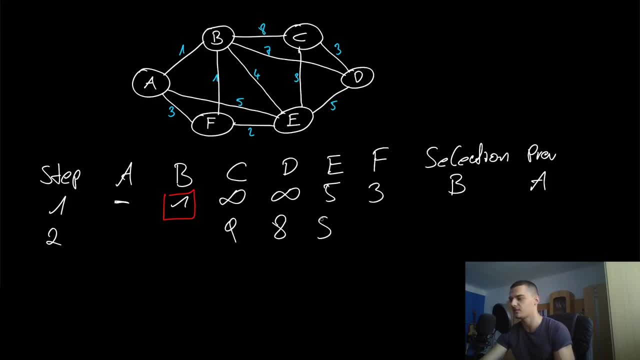 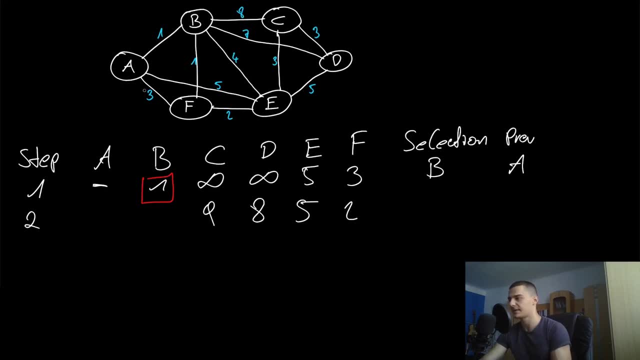 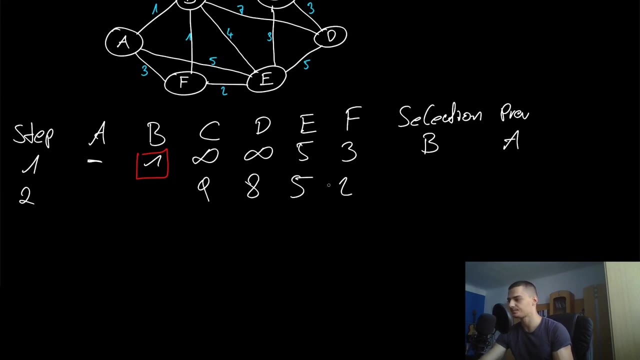 have one, or plus four, or five directly, so it's still five. we don't change anything here. and then going from a to f is a cost of two, because now instead of going directly, which costs three, we can go a, b, f, and this has a cost of two again. we pick the smallest number, which is f, um or the. 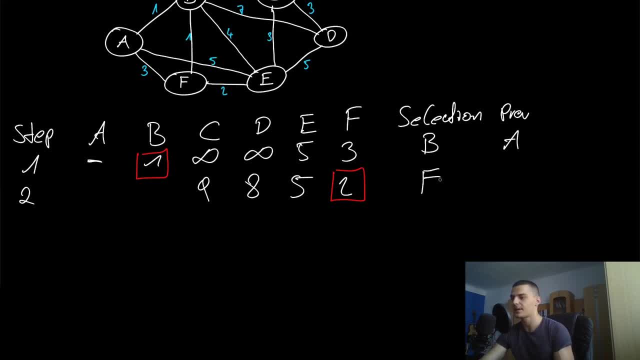 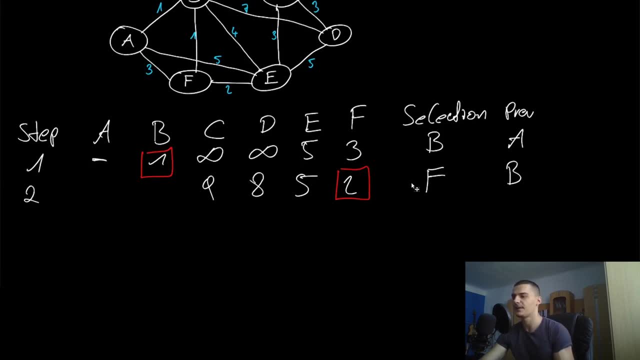 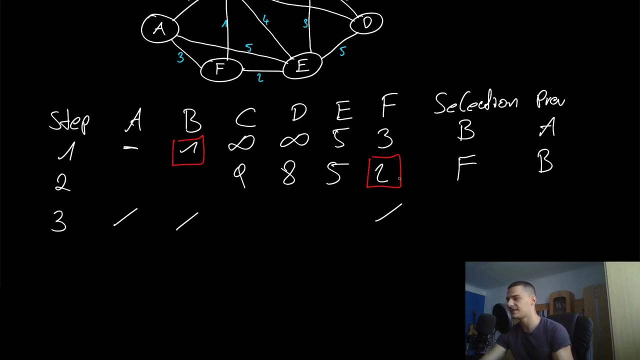 smallest cost. and then we say, okay, we selected f, but we selected it from b. we didn't select it from a directly. this is important. uh, we selected it from b. then we say three steps. uh, we ignore b, f and a, so we only care about c, d, e. 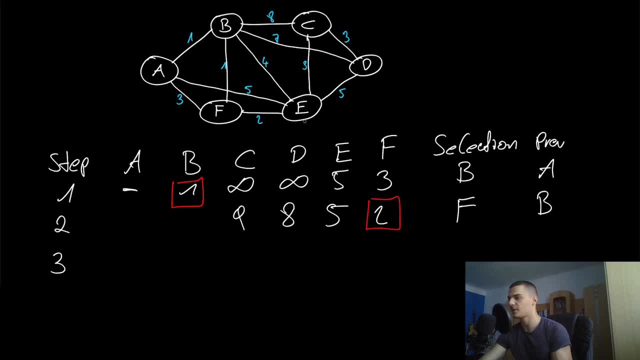 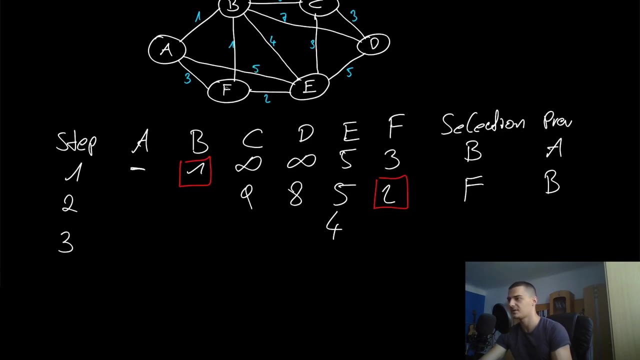 and what we do now is we ask: okay, from f going to e takes a cost of uh two. so two plus two is four, which is less than five. uh, going from f to c is not really impor, uh really possible. we cannot just go ahead and find a shorter path to c. so what? 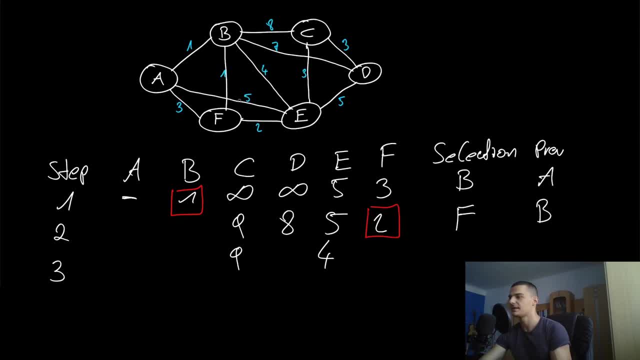 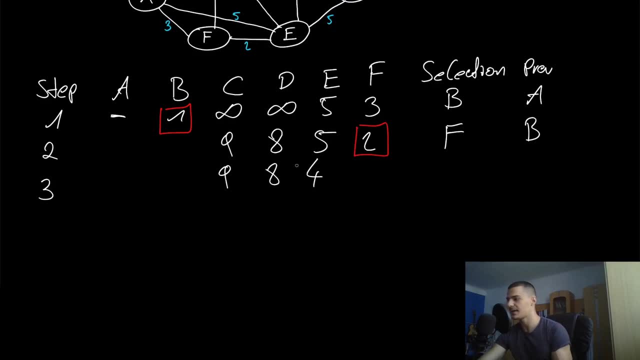 we do is we just apply that nine. it's still the shortest path that we know, and from f to d is also not possible, so we just do it like that. what we do then is we select e again, we select e from f, and then we start the next row, and now we look from e. i can access c using a cost of three. 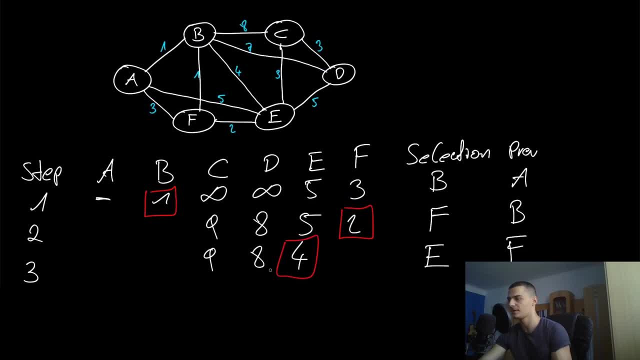 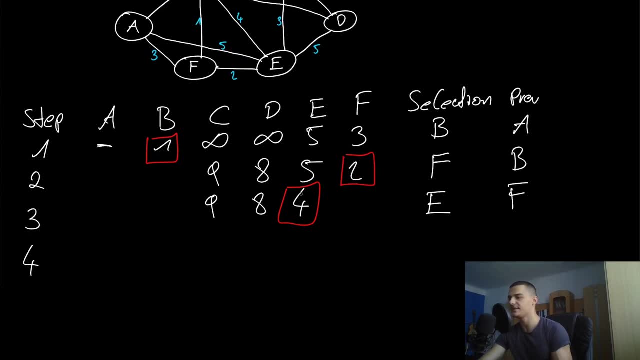 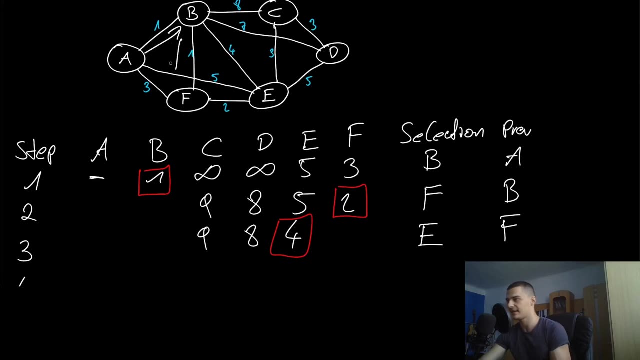 which, of course, is less than nine, because four that we already have. so you need to think about it this way. this here means that we can go from a to e with a distance of four with a cost of four. uh, this is obviously the case. if we go that, that and that, one, one, two, this is a cost of four, and 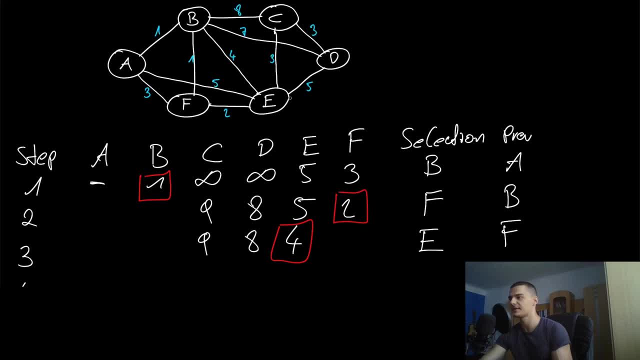 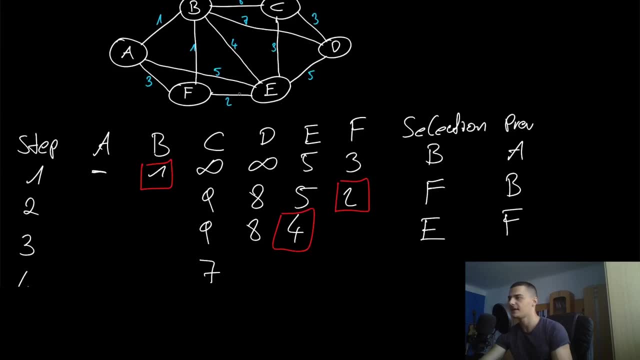 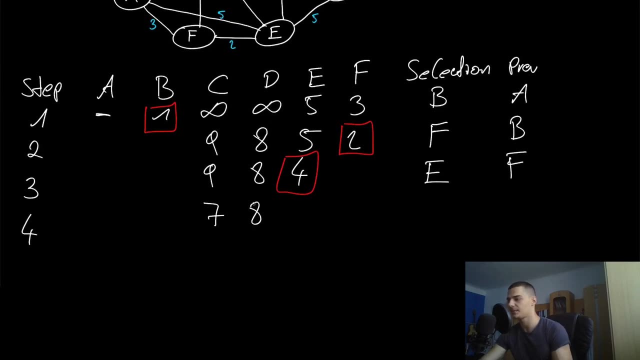 now, additionally, i can go from e to c using an additional cost of three. so this is essentially a cost of three. so we can go from e to d and to d. i have to add five. uh, in order to go from e to d, i have to add five. four plus five is nine, which is larger than eight. so we don't change that. we, uh, we. 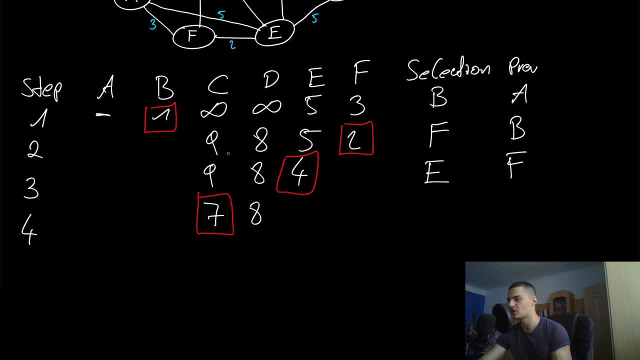 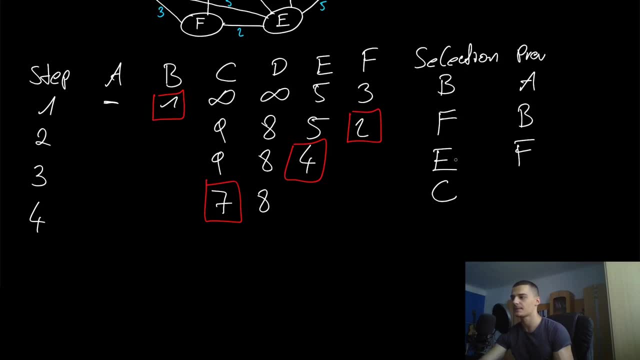 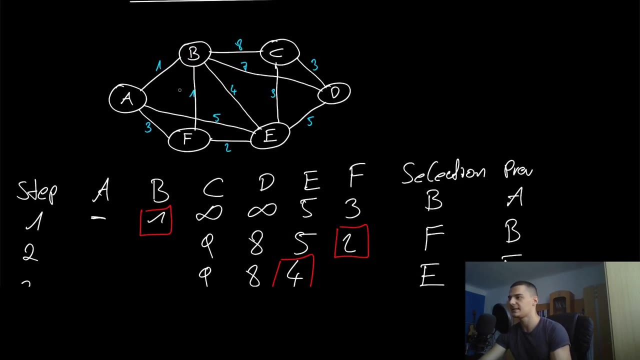 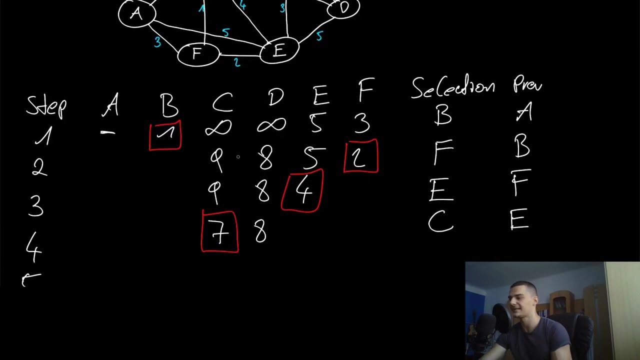 just copy the eight here and you can see that the next shortest thing is, or the next smallest number is c. so we select c, but we select c from um, from e, and then we have five steps. now we're looking at c from c. i can access d with a cost of three, which is seven plus three is um ten, so it's less, uh, it's. 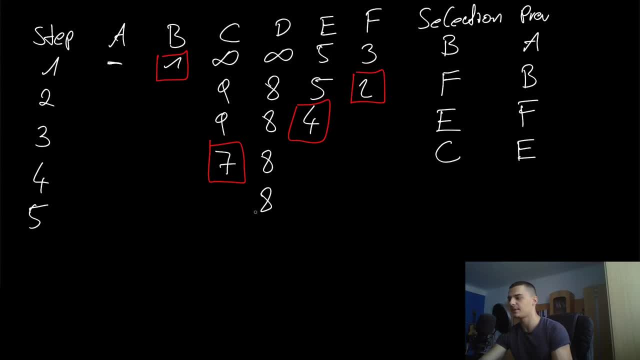 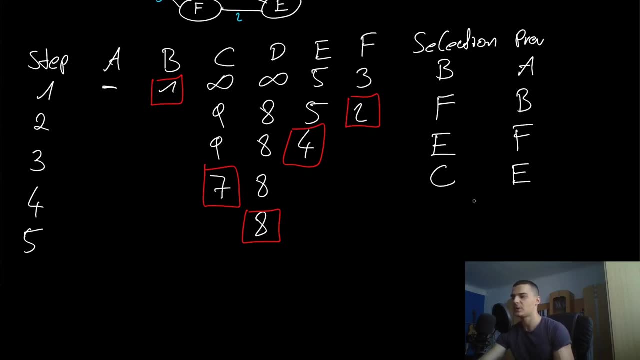 it's larger than eight, so eight is actually the smallest number. but- and this is now tricky or not tricky, but we need, you need to think about this- we're not accessing, we're selecting d, but we're not accessing d from c, because accessing it from c would have a cost of ten. so we need to ask when. 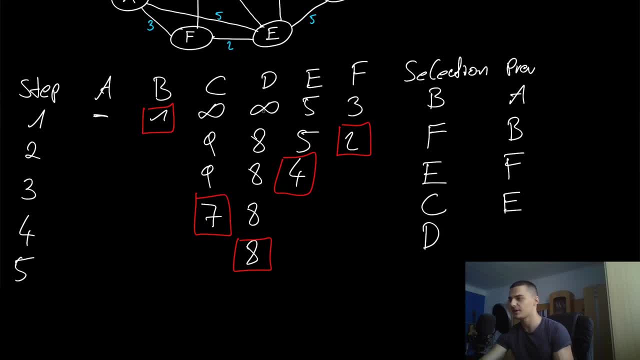 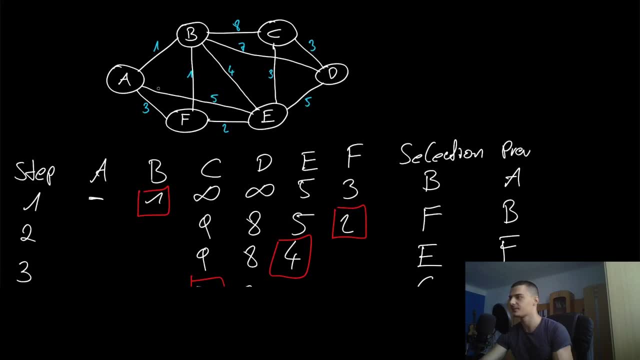 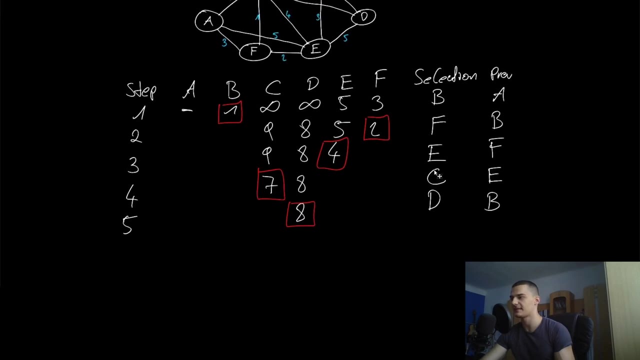 was the time where i got the cost of eight the first time. so here i got the cost of eight and i got it from b. i could access one and seven, one plus seven, so i actually access d from b, and now we can see the shortest paths in this table here. so let's try to find the shortest path from. 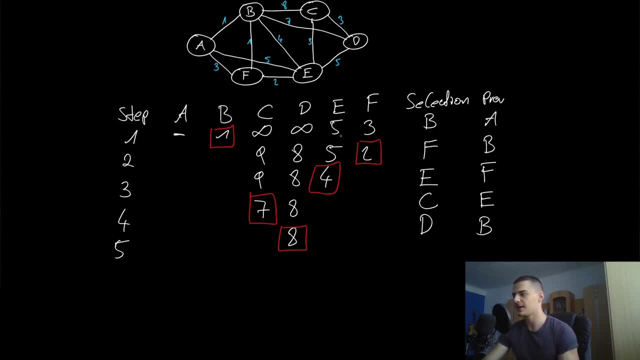 a to e. for example, if i want to find the shortest path from a to e, i just go to the column where i select e and then go back. so i can see: okay, i have to go to f, back to f essentially, then to b and then to a. so a, b. 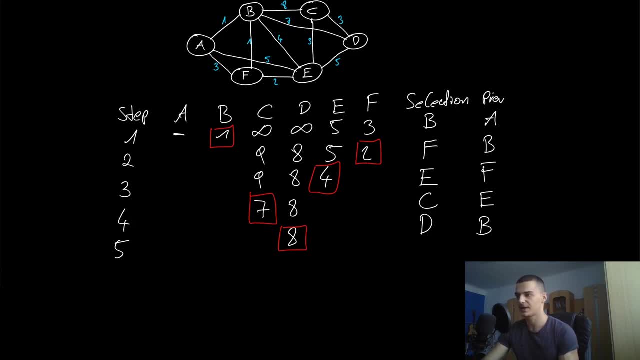 f, e is the shortest path we can. we can see it right here. um, if i want to know the shortest path from a to c, i just go c. okay, it's e, f, b, a. so it's a b, f e c, a, b, f e, c, a, b, f e c. this is the. 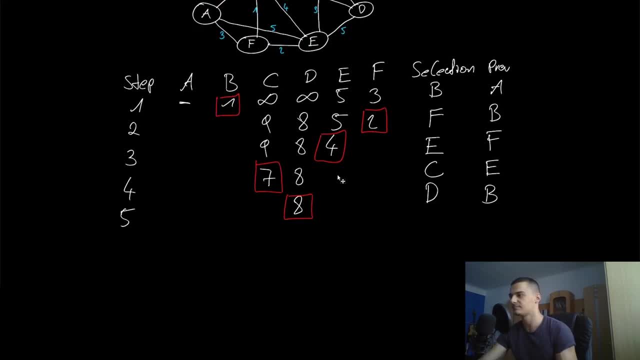 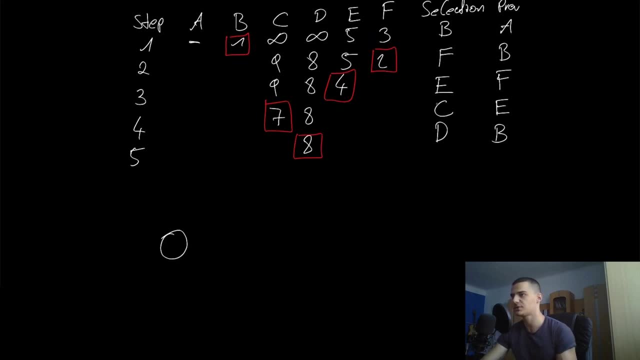 shortest path and now, if you want to have a little bit, uh, a better overview, so to say what we do is we go to f and this is the shortest path that we can see here. so we can just use these selections in previous um, this data here. essentially we can use it to graph, uh to to draw a new graph here. 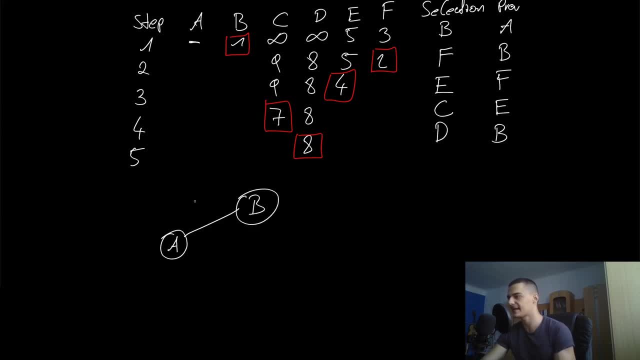 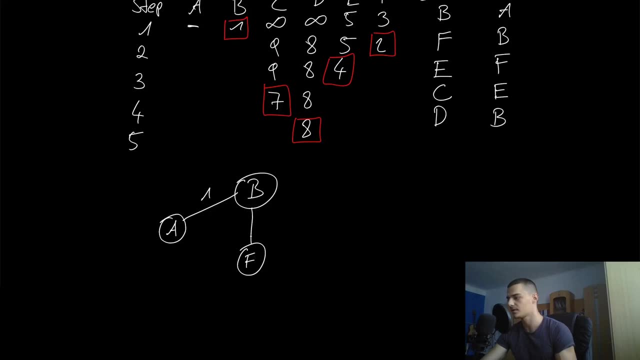 starting at a, we go to b, obviously, and this has a cost of one. from b, we go to f, and this has a cost of two, so we add one. um, then we go from f to e, and this has a cost of four, so we add two. 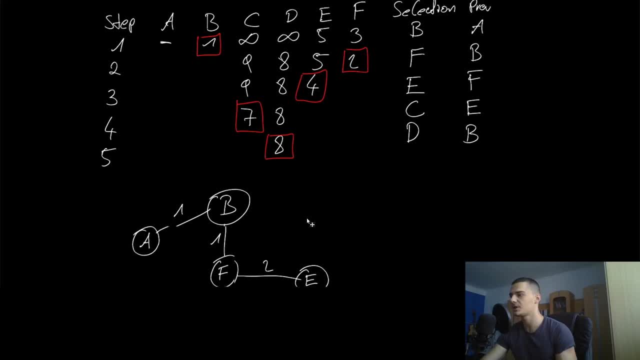 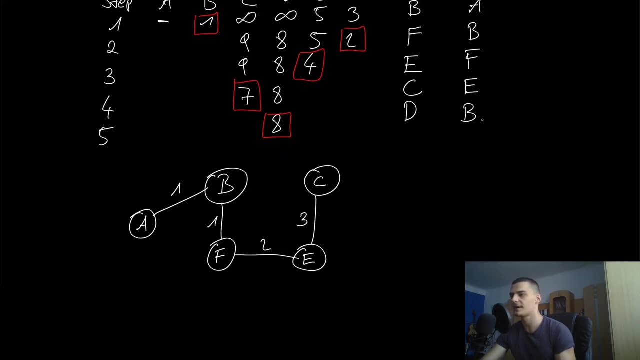 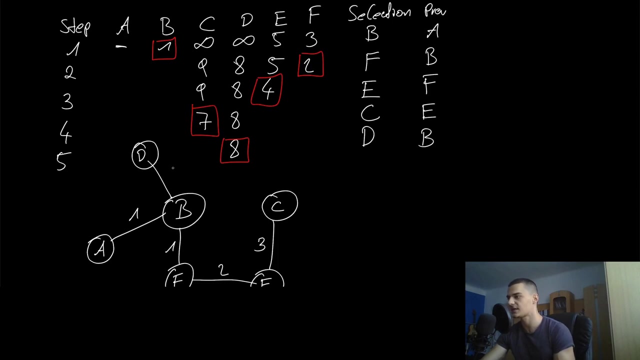 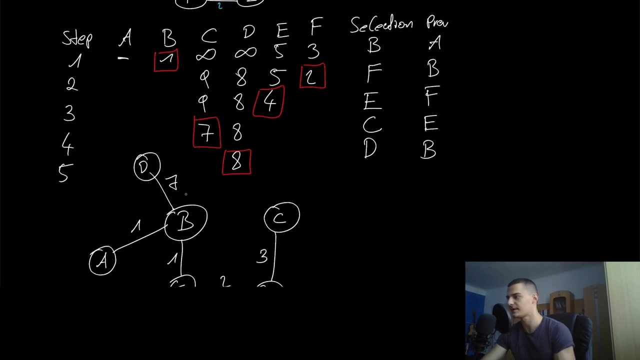 then we go from e to c, which has a cost of seven, so three more. and then we go from b to d, which means that uh, d is actually here, and this has a cost of eight. um, so this is a seven, because up until b we needed one. then this is essentially the graph. 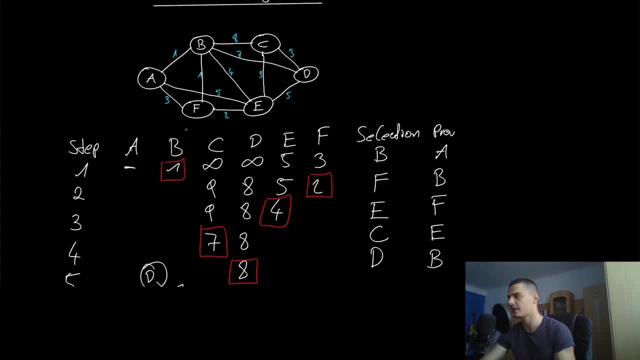 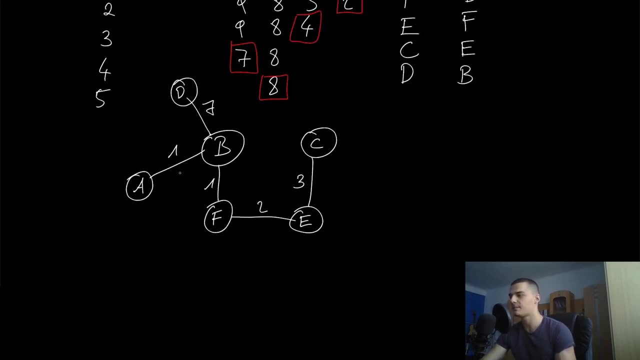 that chose us the shortest path. as you can see, it's similar to the graph above, but it's not the graph above, but all the edges that we're not using to find the shortest paths are just removed, and now we have only the most sufficient edges, so to say. now, if i want to go, 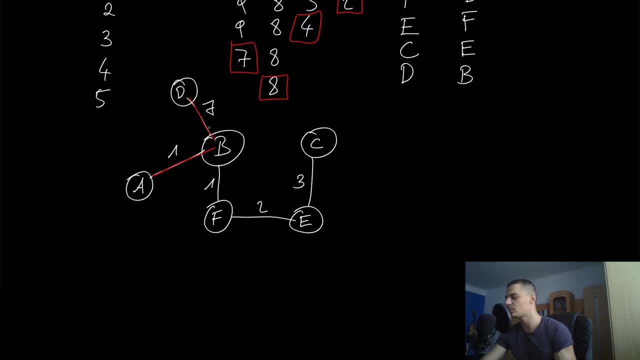 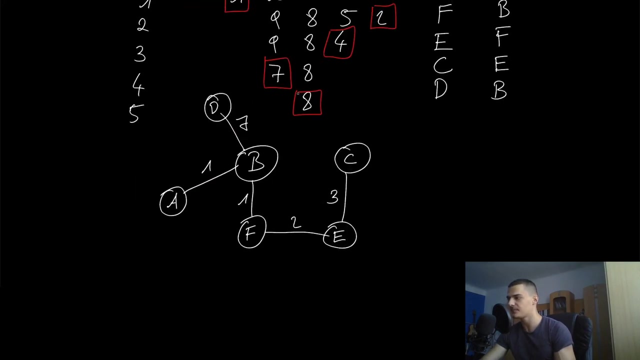 to d. i see i have to go to b first and then to d. there's only one path. this is essentially a tree, um, and it's the dike. you could say a dikstra tree, or whatever. it's just a graph showing you, um, the shortest paths to each node from a, and you can now use this to, you know, find the shortest.